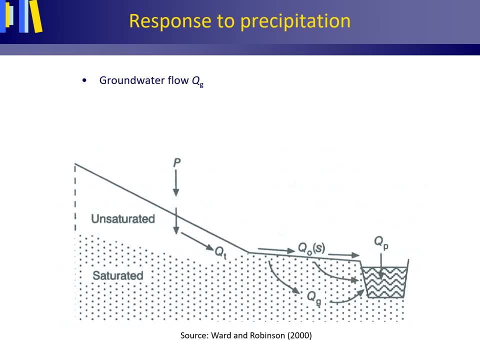 events have been observed to raise the shallow water table boyars the stream above the water level of the stream, causing groundwater flow to contribute to the stream flow. Also, during rainfall events in parts of the Netherlands with shallow water tables, groundwater may be transported rapidly through drains and ditches if these are deep enough to cut the rising water. 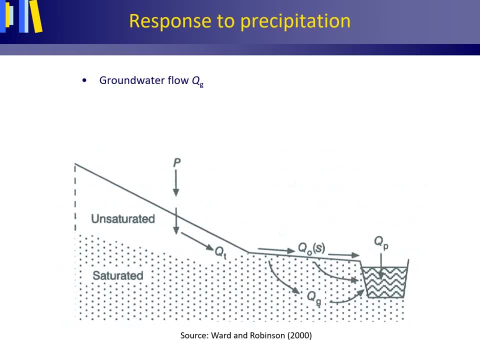 table. When a coarse textured layer with a high hydraulic conductivity overlies a fine textured layer with lower hydraulic conductivity, the percolation capacity, which is the maximum rate at which water can percolate through a soil, is initially controlled by the coarse textured layer. However, when the wetting front reaches the fine textured layer, 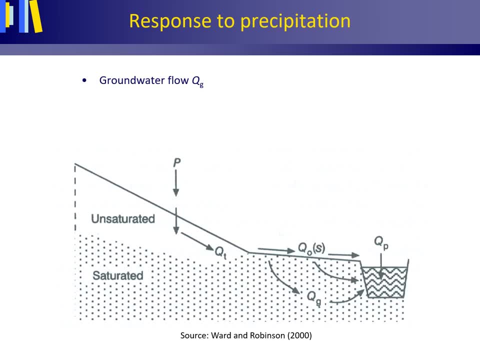 the percolation capacity will be controlled by the fine textured layer and will drop sharply If percolation continues. a purged water table may develop in the coarse soil above the impeding layer, which, in sloping terrain, may result in throughflow. Subsurface soil water flow parallel to the land. 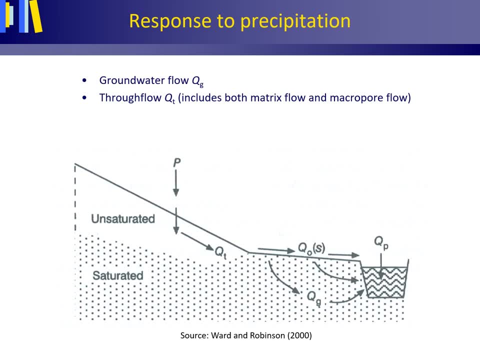 surface in the direction of the stream or water course. If the quantity or volume of rain in millimeter causes the storage level in millimeter to increase and then to exceed the water storage capacity of the soil in millimeter, water is forced to the surface where such a purged water. 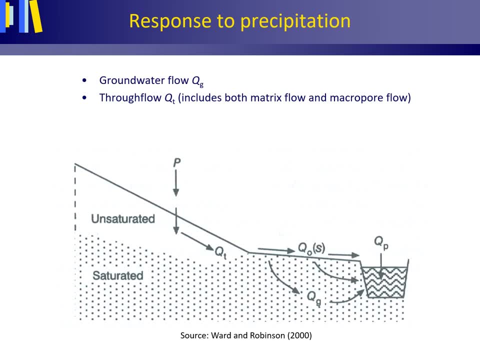 table cuts the sloping land surface and then drop to the surface which is in the middle of the stream, water will flow over the land surface as overland flow, Because the overland flow stems from the upper soil profile being saturated. overland flow produced this way is called saturation excess. 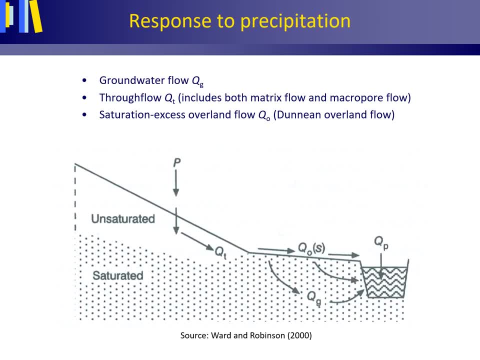 overland flow or in short, saturation overland flow. in Dutch verzadigings overland flow, Saturation, excess overland flow is sometimes referred to as Dunnian overland flow after Thomas Dunn, professor in geomorphology and hydrology. This type of overland flow is fundamentally 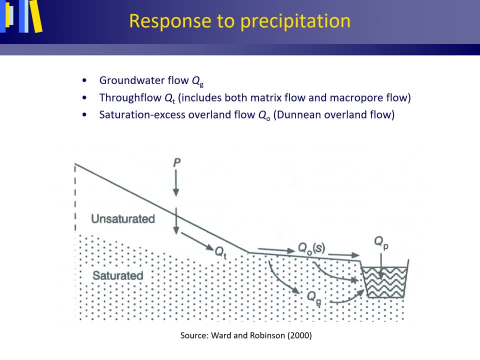 different from an earlier discussed type of overland flow where the rainfall intensity in millimeter per hour exceeds the soil's infiltration rate in millimeter per hour, as can be observed on bare or crusted surfaces with reduced infiltration Under arid or semi-arid climates. this type of overland flow is called infiltration excess. 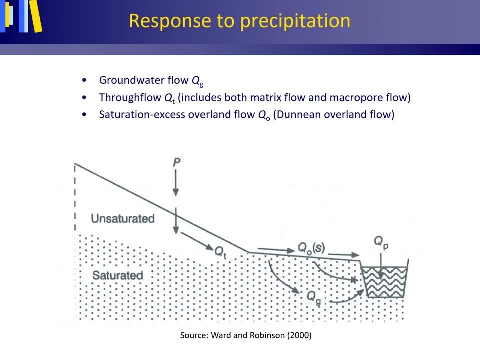 overland flow, or Hortonian overland flow after the earlier mentioned American ecologist and soil scientist, Robert E Horton. Macropores are pores with a diameter larger than 30 micron and relate to porosity around soil aggregates, Special type of both throughflow and macropore. flow is the macropore of the soil. This is the macropore of the soil, which is the macropore of macropores. This is the macropore of the soil, which is the macropore of the soil. 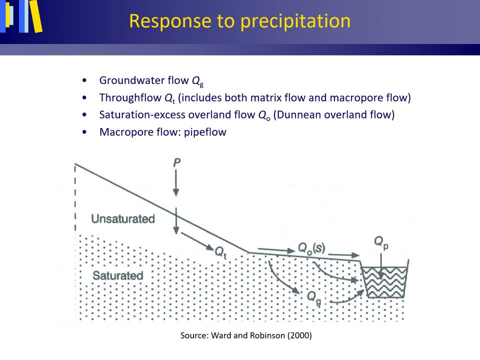 The third type of overland flow is pipe flow. Pipe flow is rapid throughflow bypassing the soil matrix, for instance when water flows through burrows made by moles or voles or when it flows through artificial drains. Soil pipes are a special type of macropore. 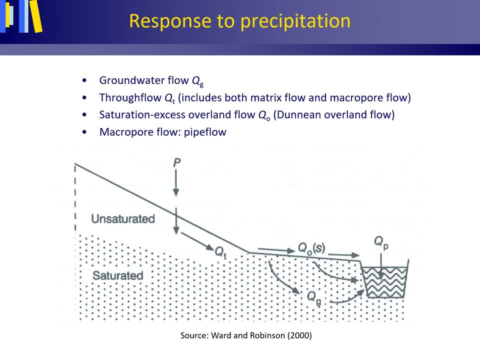 as they are continuous and prolonged in one direction: parallel to the land surface. During wet conditions, natural soil pipes, mole and vole burrows may rapid transport water parallel to the land surface in the direction of streams. During dry conditions, natural soil pipes located near the land surface and above the water table contain little or no. 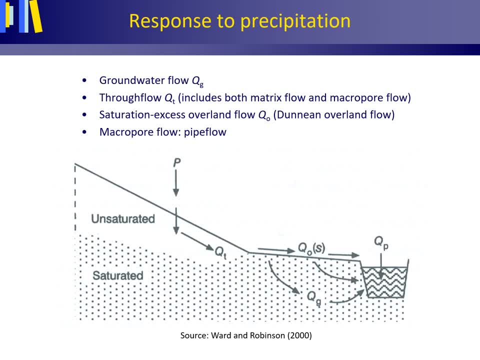 water. Water can only enter a soil pipe from its surrounding soil matrix if in the matrix, a critical threshold suction related to the natural soil pipe's diameter is reached, As the natural soil pipe's diameter of a mole or a mole is greater than the diameter of the natural soil pipe's diameter. 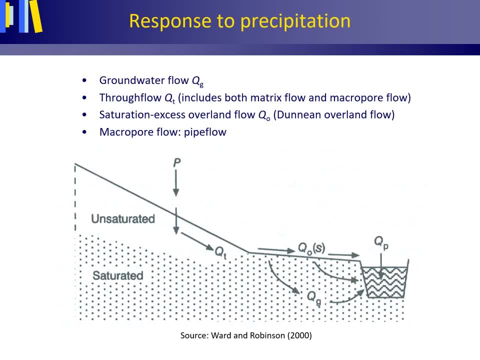 or a vole burrow is in the order of 1 to 2 cm, the matrix threshold suction must be almost 0 cm, meaning that the surrounding matrix must be near-saturated. Similarly, artificial drainage pipes, for instance, used to drain cultivated land, are only effective when the 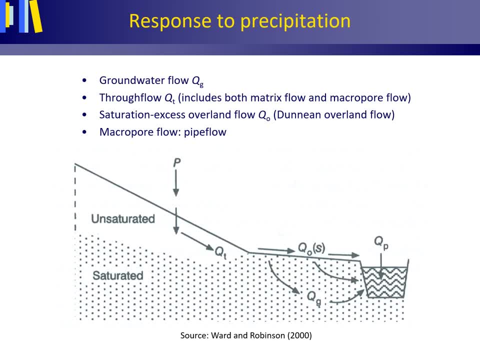 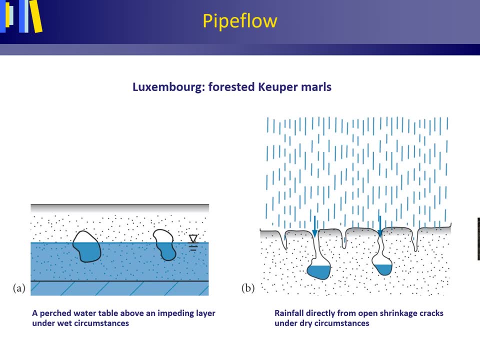 soil matrix is near-saturated or when the water table rises to the level of the drainage pipe. This sheet shows a schematic presentation of two different ways for the occurrence of pipe flow. The illustration to the left shows the situation where water is fed to a pipe from a purged 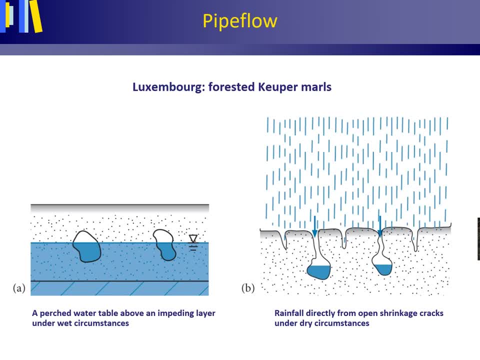 groundwater body that has developed above an impeding layer. This is the situation where water is fed to a pipe from a near or fully saturated soil matrix next to the pipe. The illustration to the right, on the other hand, shows the situation of water being fed from pipe flow to a pipe from the 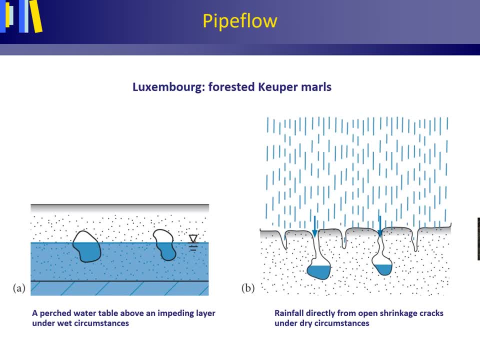 shows a situation where pipe flow develops under dry circumstances. In soils prone to seasonal shrink swell, such as clay soils, the occurrence of dry circumstances or thaw after a freezing period can cause shrinkage cracks to open, If the shrinkage cracks are deep enough and connect with the pipes. 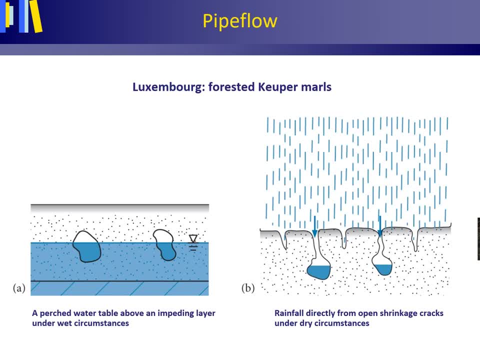 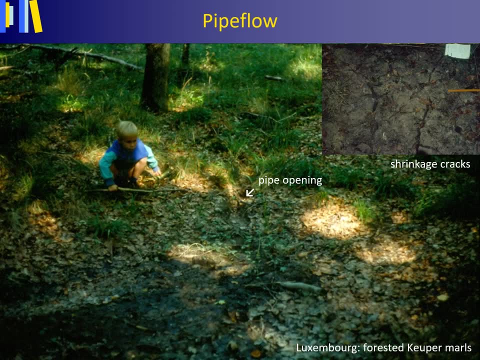 a very rapid short-circuiting of rainfall via shrinkage cracks and pipes to a downslope stream can evolve. As an example, soils in forested areas of the Steinmeer-Gokuiper miles in the Gutland of Luxembourg are made up of a 30 cm thick loam textured layer. 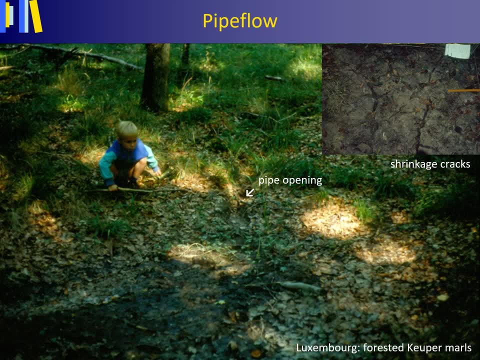 overlying an impeding clay horizon. The topsoil above the impeding layer contains many mole burrows that are interconnected in a downslope direction for observed lengths of up to 120 m and that support the short-circuiting action just described during a large part of the year. 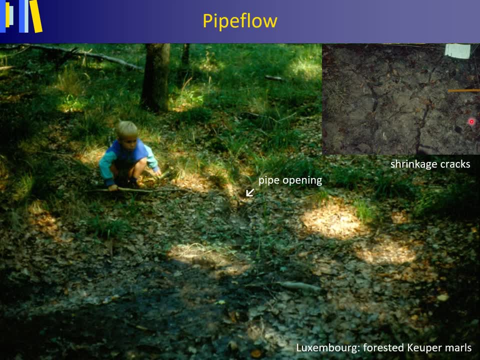 When shrinkage cracks are open, as shown here and connected with these natural pipes. Water has been observed to gush out of pipe openings at downslope near stream positions in these forests during many storm events in the area, and subsurface flow through the pipes was observed as turbulent and erosive. 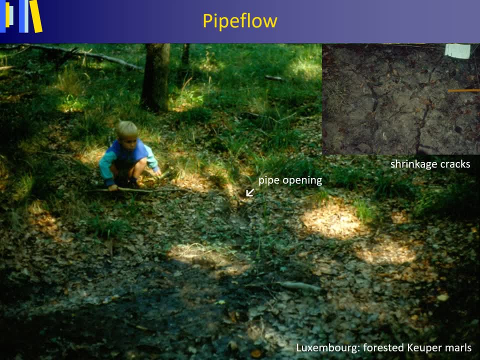 further enhancing its short-circuiting action. One such pipe opening is indicated on this photo. The area of sedimentation on leaves lying on the forest floor from water that has gushed out of this pipe opening is clearly visible as a darker area on the photo. 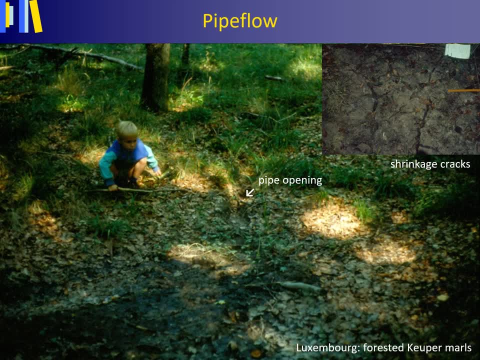 Shrinking and swelling of clay is a seasonal phenomenon and, interestingly, for every dry period, these shrinkage cracks in the Steinmerker Korpel miles of Luxemburg, can be observed to reappear at the exact same spot as before. 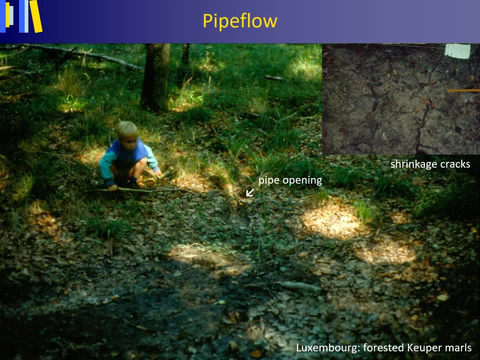 Similarly, subsurface flow through artificial drainage pipes in a clay soil in Oxfordshire, England, was found by Robinson and Bevan to be more responsive to storms in summer than winter, also because in summer the soil was dry and dry and cracked. 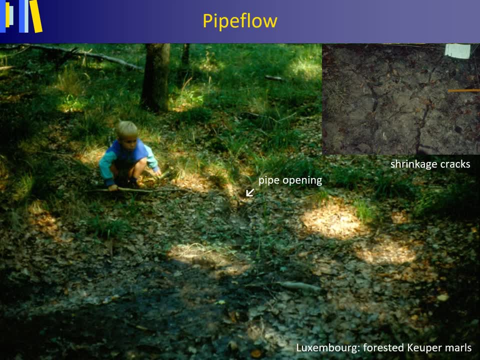 The relative importance of matrix flow and macropore flow generally depends on rainfall intensity and duration, infiltration capacity of the matrix, the shape and connectivity of pores and the wetness of an area prior to rainfall, the so-called antecedent moisture content. 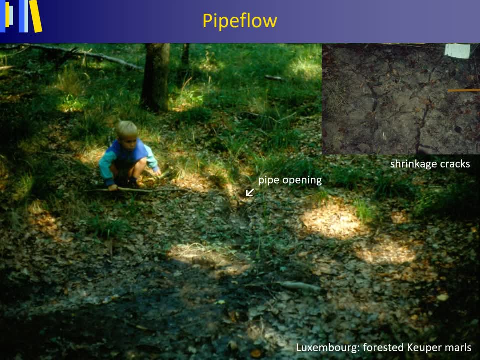 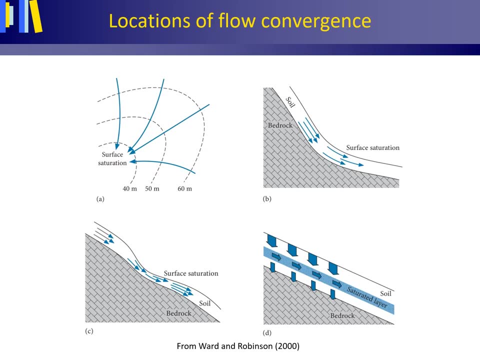 but is also linked to topographical position in the landscape and vegetation. This sheet shows principal locations of flow convergence in drainage basins. Infiltration into a layered soil may lead to the development of a purged water table, Importantly for humid climates. 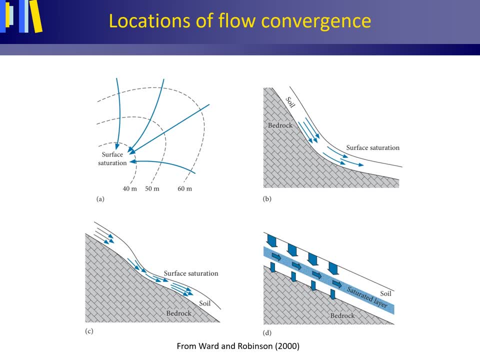 when the purged water table reaches the land surface, any extra rain that falls will immediately become saturation, excess overland flow, which is transported over land and thus rapidly to the stream, contributing to the quick flow of the stream. Topographic convergence zones can be hillslope hollows or topographic depressions. 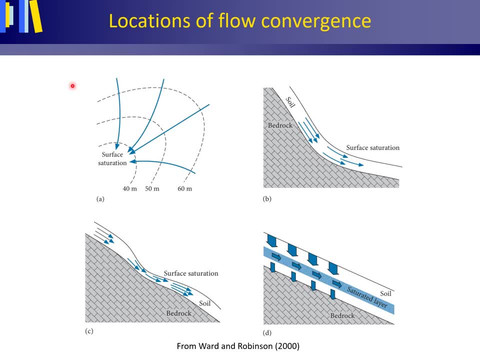 that is, slope concavities in plan or slope concavities in section, as shown in this figure under A and B, For both types of concavity, throughflow can enter such a concavity more rapidly than it can leave downslope. 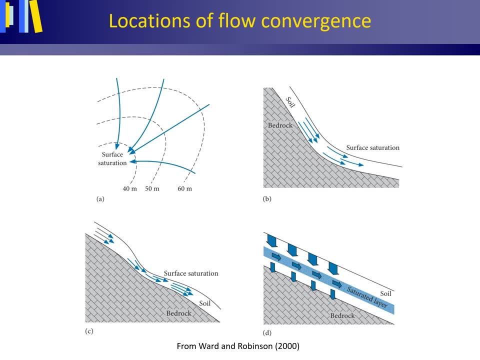 thereby forcing water to the surface. Also, where an upper layer in the soil that supports throughflow becomes thinner, a purged water table may develop and rise to the land surface, as shown under C. A purged water table and throughflow may also develop. 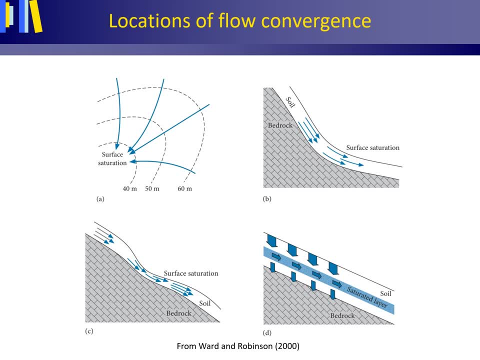 as the result of the reducing hydraulic gradient as water moves downward through a soil, even a relatively uniform one, This may cause the development of a saturated layer at some depth in the soil profile, as shown under D. In conclusion, the process of a rising water table reaching the land surface. 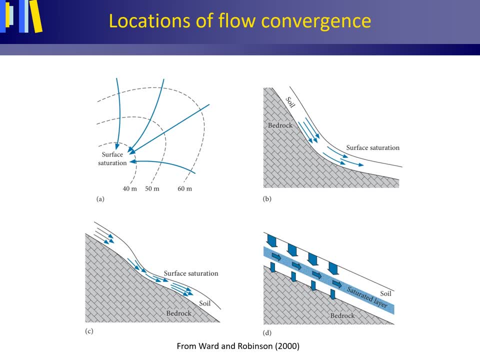 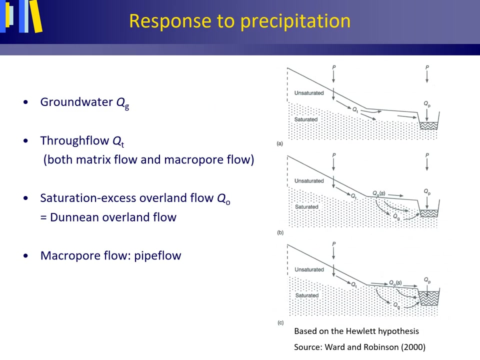 is a very important mechanism for the generation of saturation: excess overland flow in humid climates. The saturated areas where quick flow is generated, with saturation often occurring from below, as just explained, are called variable source areas or partial areas. This figure provides a summary of the Hewlett hypothesis. 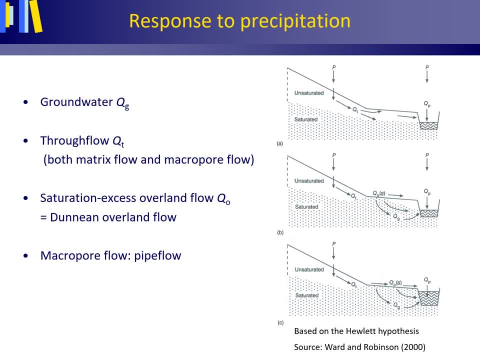 of runoff formation in humid climates, as presented by Ward and Robinson. Figure A shows that water infiltrates the slope surface and moves its throughflow, that is, matrix flow and or macropore flow, under the slope surface. Figure B shows that 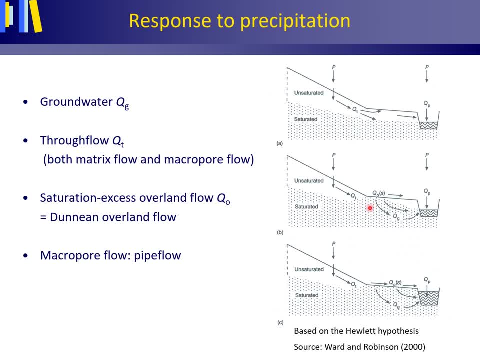 convergence and infiltration in the lower slope areas leads to surface saturation and groundwater recharge, which will create both an overland flow and a groundwater flow contribution to the stream, with the groundwater ridge expanding in some locations into a wider area of surface saturation. 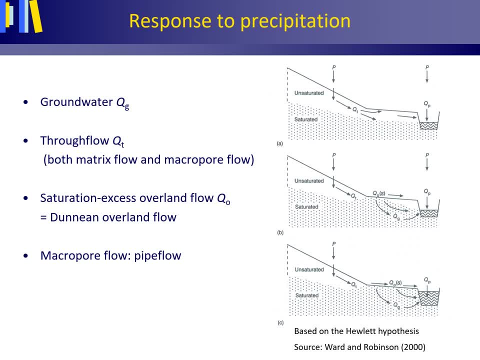 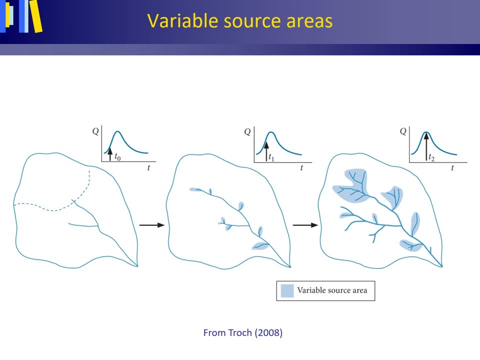 as shown in Figure C. This figure shows that the areas that become saturated from below expand, upslope and upstream if rainfall continues. This phenomenon has been observed in situ as well as through remote sensing techniques. These saturated areas that contribute to quick flow can expand and contract in size between storms. 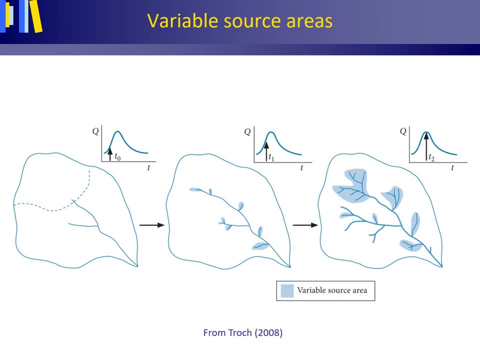 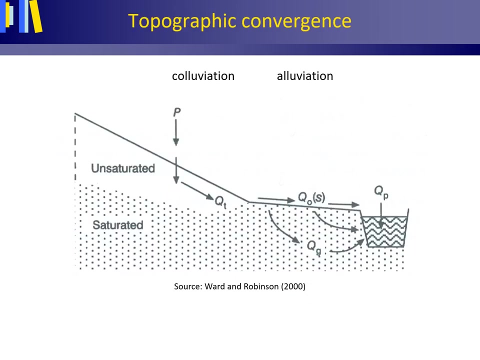 and during the course of a single storm. They are called variable source areas, Source areas with as adjective variable because of its expanding and contracting nature. Often, but not necessarily so, variable source areas are located near the channel network that drains the area. 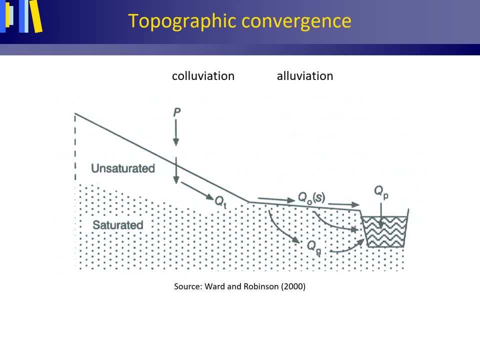 The latter has to do with processes such as colluviation- the deposition of sediment through the action of gravity at the foot of a slope, causing the hillslope angle to diminish in the direction of the stream- and alluviation- the deposition of sediment by streams. 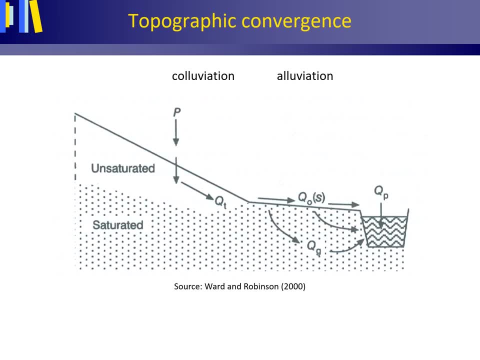 causing areas near the stream to be flat, that is, when viewed in cross-section. These flat areas are called alluvial terraces and their slope, logically, is parallel to the former stream's gradient. Thus processes such as colluviation and alluviation. 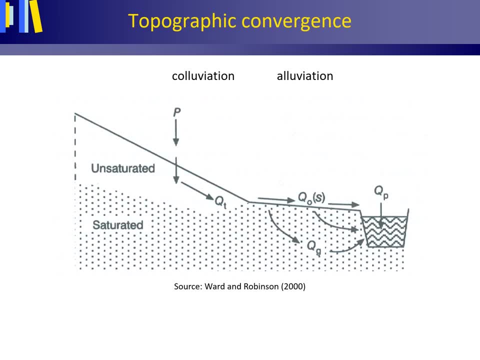 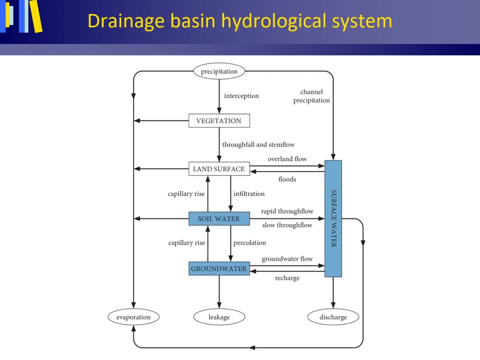 are responsible for having flattened and or flattening the foot of hillslopes and thus for topographic convergence that amplifies the effect of a rising water table and may cause throughflow to exfiltrate. This sheet shows the earlier presented drainage basin hydrological system. 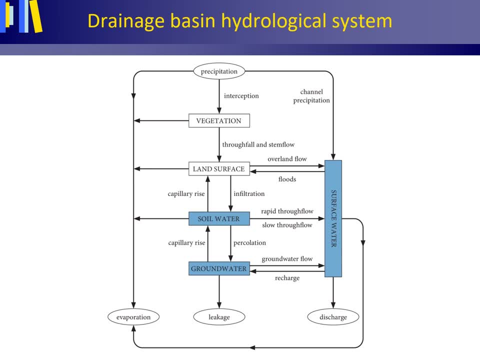 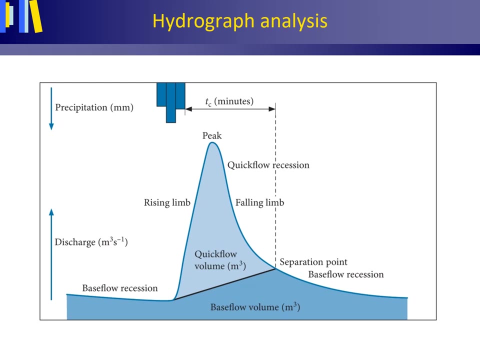 but now with the processes between the main water compartments discussed at this and preceding lectures more prominently included. This figure shows a hydrograph, a graph of the changes in discharge along the vertical axis, the time along the horizontal axis for a precipitation event, together with the number of hydrological terms. 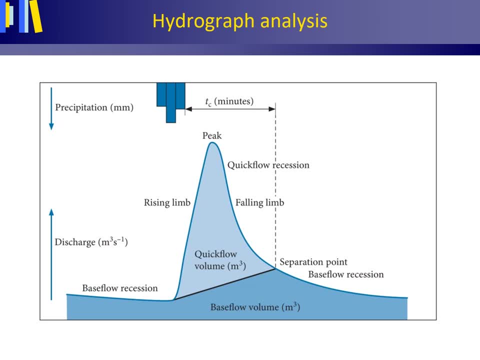 used to describe a hydrograph. The discharge or part of the discharge of a stream caused by processes delivering water rapidly to the stream is called quickflow. For the discharge volume that stems from these rapid processes, we use the term quickflow volume. 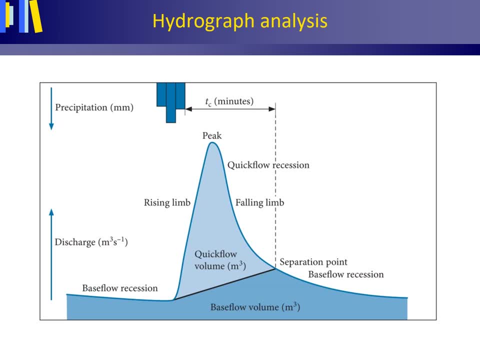 During periods with no precipitation, many streams, especially in humid areas, continue to carry water. The streams are fed by processes such as sustained groundwater flow and slow throughflow through the soil matrix from an earlier precipitation event or events, The discharge or part of the discharge. 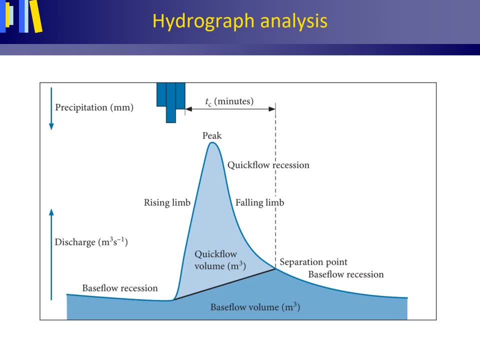 of a stream caused by processes delivering water slowly to the stream is called baseflow. For the related discharge volume we use the term baseflow volume. The rising limb is part of the hydrograph, with increasing discharge before the hydrograph has reached its peak. 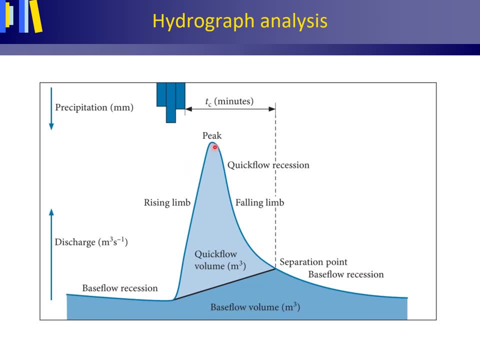 the peak being the maximum discharge during a precipitation event. The falling limb is part of the hydrograph. with decreasing discharge after the hydrograph has reached its peak, The term recession curve is synonymous to the falling limb. The quickflow recession is part of the hydrograph. 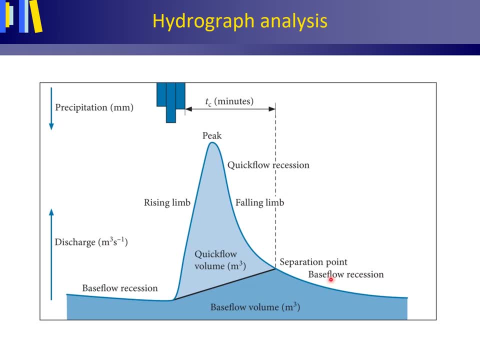 with gradually declining quickflow. The baseflow recession is part of the hydrograph with gradually declining baseflow. Separation point is the point on the recession curve that separates the quickflow recession from the baseflow recession. Inflection point is the separation point. 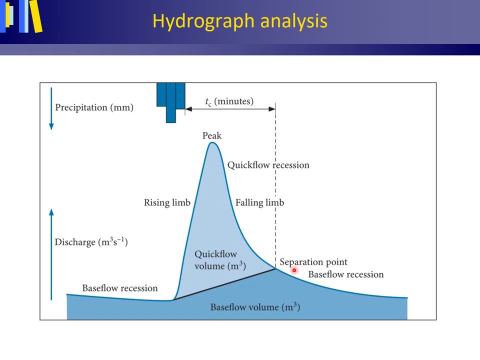 determined by assuming that the recession curve can be modeled as the discharge from linear reservoirs that represent quickflow and baseflow. More on this shortly. Finally, the time of concentration is the time required for surface water or other water contributing to the quickflow of a stream. 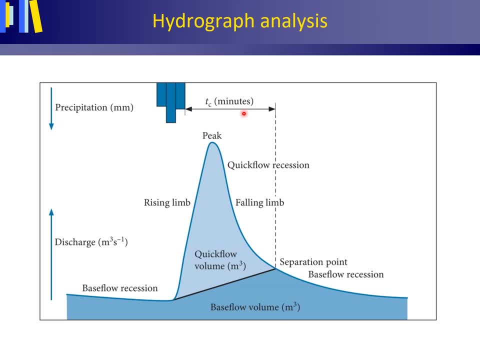 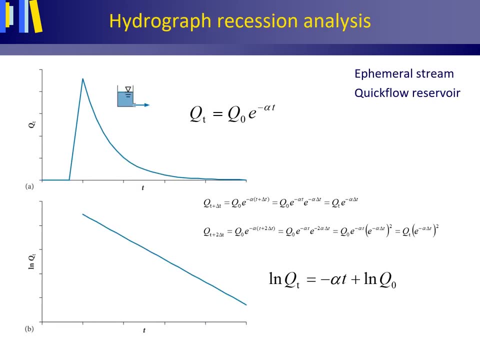 to flow from the farthest point in the watershed to the outlet. Streams that hold water throughout the year are called perennial, whereas a channel that only holds water during and immediately after a rain or snowmelt event is called ephemeral. An ephemeral stream thus has no baseflow. 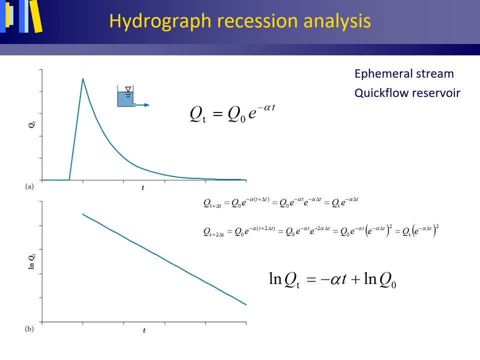 only quickflow. This sheet shows a hydrograph of heavy rain on a wadi, a usually dry riverbed in a semi-arid climate, with the exception of periods during and shortly after heavy rainfall. A wadi, thus, is a type of ephemeral stream. 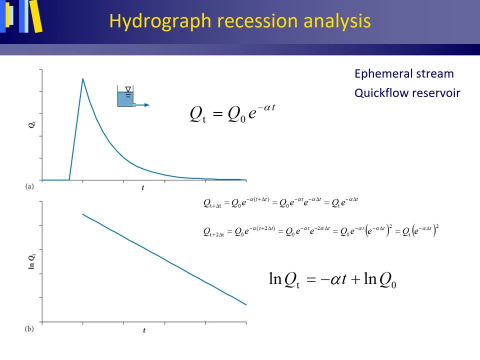 and its discharge is made up solely of quickflow For an ephemeral stream. the recession curve can conceptually be interpreted as outflow from a quickflow reservoir. The recession curve can mathematically be described as an exponential decrease starting at the hydrograph peak. 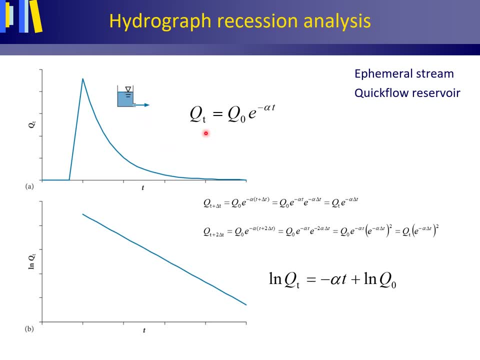 as shown here. Qt is discharge at time t after the start of the recession, in cubic meter per second. Q0 is discharge at the start of the recession in cubic meter per second. thus, at the hydrograph peak, t is zero seconds. E is the base of natural logarithms. 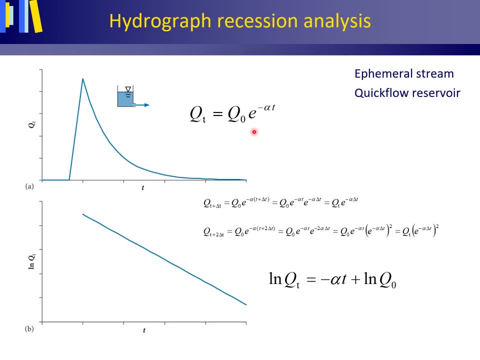 2.71, etc. Alpha is the recession constant per day and t is time in days. In analogy with the Horton equation for pondered infiltration, the equation can be rewritten for small constant time intervals, delta t, as shown here and here. 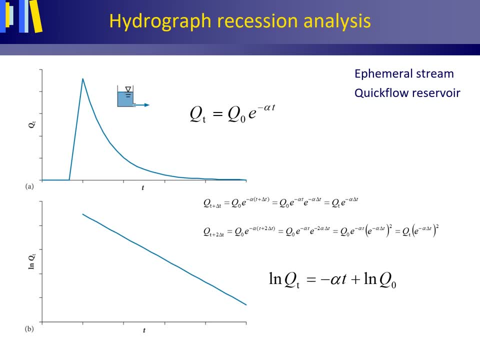 Remarks made for the decay constant alpha when introducing the Horton equation for pondered infiltration. similarly hold for the recession constant alpha. in these equations, E to the power minus alpha, delta t is smaller than one. Also, if the recession constant alpha is large, the recession curve shows a steep decline. 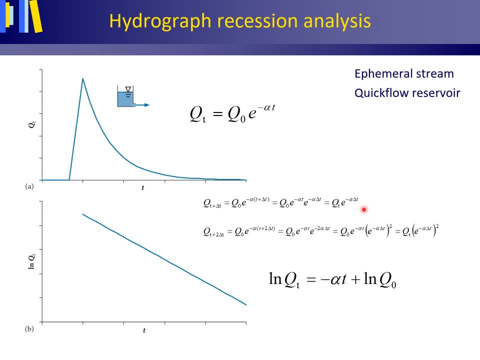 and the depletion of the reservoir is fast. Consequently, if alpha is small, the recession curve shows a slight decline and the depletion of the reservoir is slow. Alpha ranges from one thousandth per day for deep groundwater to over three per day for overland flow. 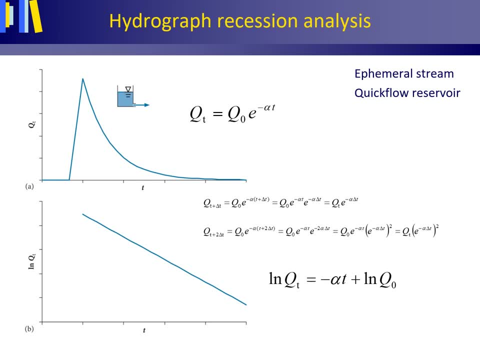 The equation can be rewritten in semi-logarithmic form, as shown here. This equation plots as a straight line in a graph, with ln on the vertical axis and t on the horizontal axis, and the value of alpha can simply be determined as the absolute value of the slope. 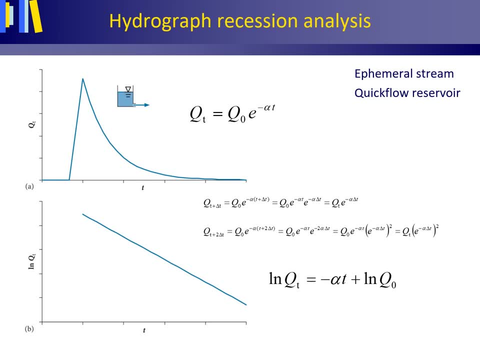 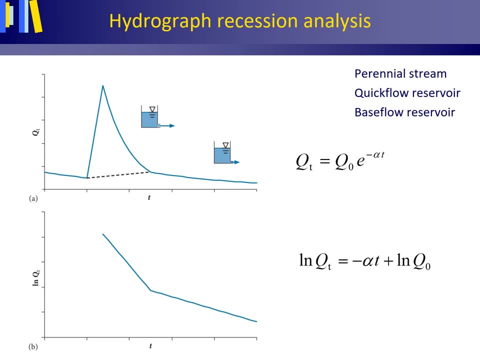 of this straight line. This sheet shows the hydrograph of a perennial stream, for instance, a stream in a humid climate setting. The discharge of the perennial stream is made up of both quick flow and base flow. The recession curve of the hydrograph. 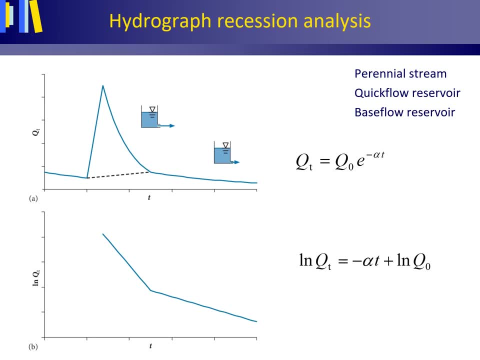 shown here can conceptually be interpreted as outflow from both a quick flow reservoir and a base flow reservoir, with the larger outflow per unit of time from the quick flow reservoir. At the separation point the quick flow reservoir has emptied and from then on. 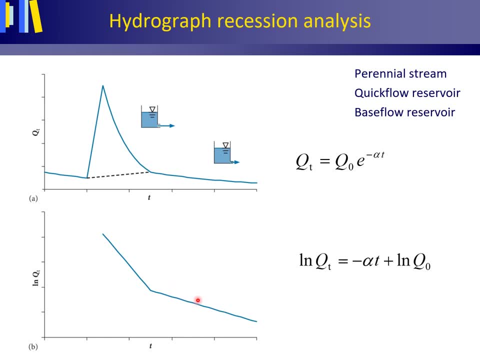 there is only outflow from the base flow reservoir. As the outflow from the quick flow reservoir is dominant, the first part of the recession curve after the hydrograph peak can simply be interpreted as outflow from the quick flow reservoir alone. The recession curve. 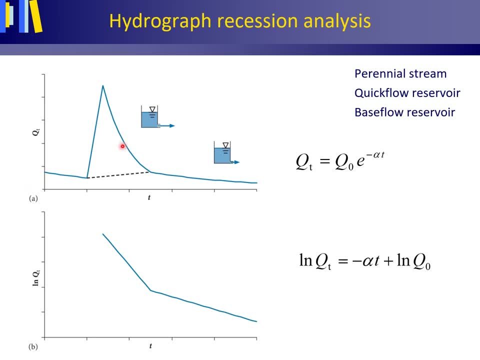 can therefore mathematically be described as first an exponential decreasing outflow from the quick flow reservoir and then, after the separation point, an exponentially decreasing outflow from the base flow reservoir. For both parts of the recession, the just discussed equations can be used. 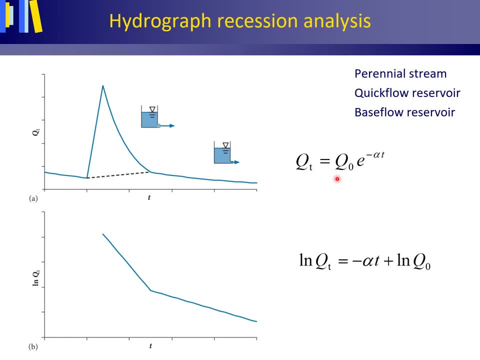 be it with a different value of the recession constant alpha for the quick flow and base flow reservoir. Note that the quick flow reservoir has been drawn with a larger opening at the bottom than the base flow reservoir. The size of the opening and the friction are incorporated. 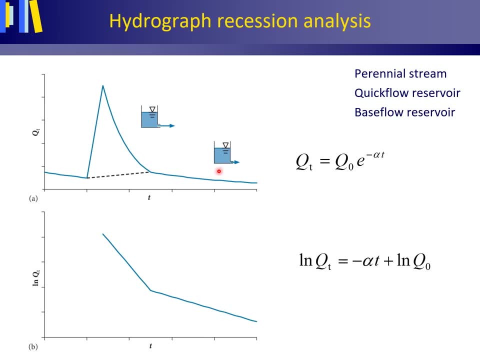 in the value of the recession, constant alpha, alpha being largest for the quick flow reservoir with its fast depletion. The figure shows a base flow separation line obtained using the constant slope inflection point method. The position of the inflection point is found as the point in time. 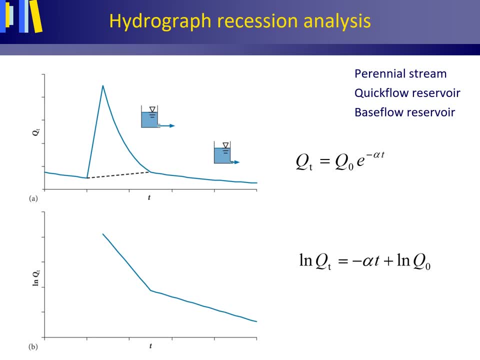 where the slope of the semi-logarithmic plot of ln versus t changes. The method has been extensively used by me when comparing hydrographs of brooks in small 1 to 2 square kilometer forested and grassland drainage basins in the Kuiper miles of Luxembourg. 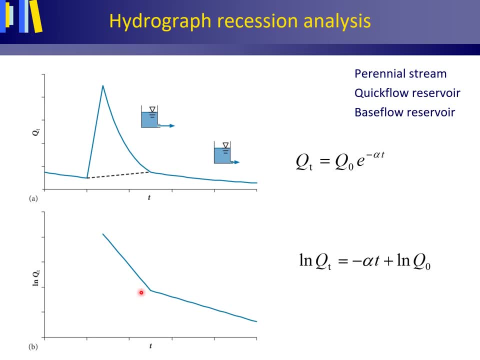 Because usually more than one inflection point is found on a recession curve, I use the inflection point with the lowest discharge as the selected inflection point to distinguish between quick flow and base flow. There are many methods for hydrograph separation into quick flow. 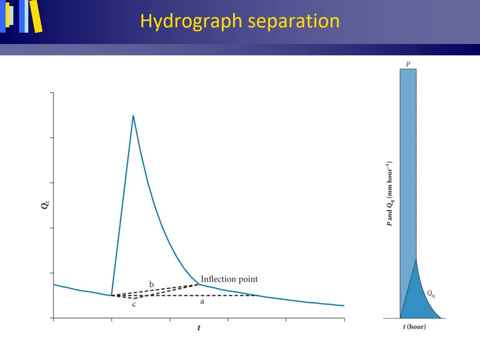 and base flow. All methods have in common that they are unavoidably arbitrary. Importantly, one should always stick to the method one sets off with when analyzing hydrographs, or else the comparison basis is lost For all methods. the area under the hydrograph curve. 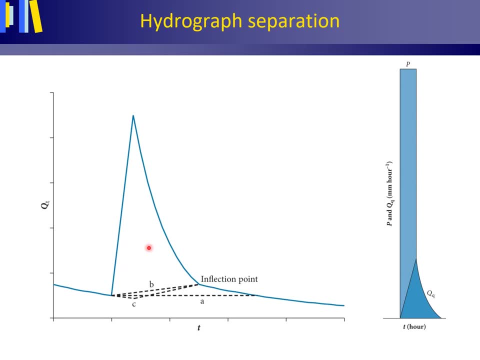 but above the base flow separation line or curve gives the quick flow volume during the precipitation event in cubic meter, whereas the area under the separation line or curve gives the base flow volume in cubic meter. There are many methods of hydrograph separation. This sheet shows. 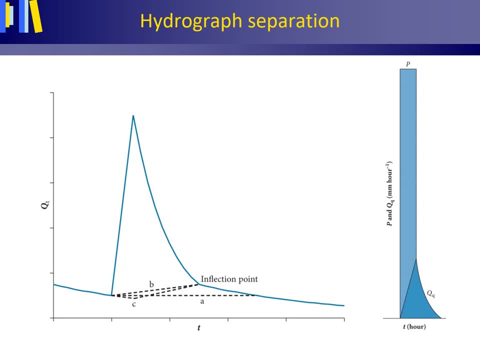 three graphical methods. The constant discharge method A assumes that base flow during a precipitation event is constant and equal to the discharge level at the start of the precipitation event. A large disadvantage of this method is that the discharge may not return to this starting level because of the start. 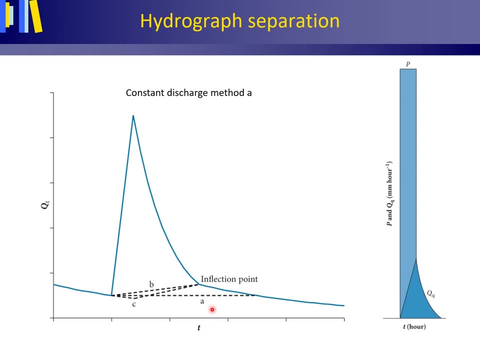 of a new precipitation event. The constant slope inflection point. method B assumes that the base flow during a precipitation event- used by me- assumes an immediate response in base flow to precipitation and connects the start of the rising limb with the inflection point on the recession curve. 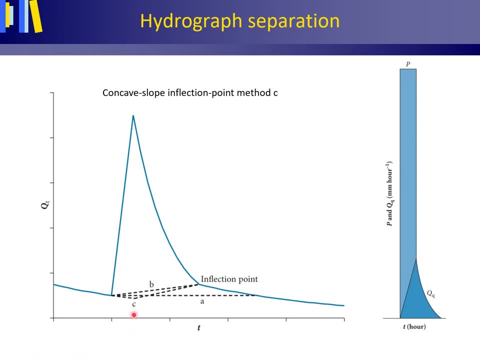 The concave slope inflection point. method c assumes a continued decrease in base flow during the rising limb of the hydrograph and projects the declining antecedent base flow recession prior to the precipitation event directly under the hydrograph peak. the minimum obtained this way is then connected to the lowest inflection point on the recession curve. 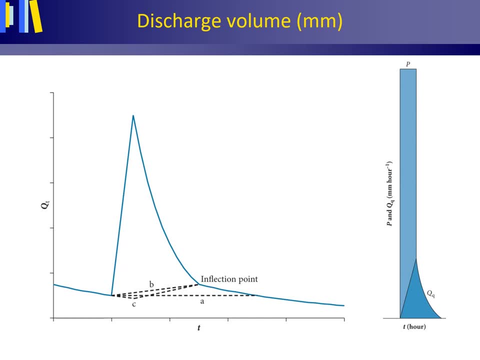 Similar to precipitation depth and evaporation. the discharge volume of a river may be presented as a length unit. for instance, millimeter discharge volumes in cubic meter can simply be converted into millimeters to meter by dividing by the total drainage basin area in square meter. 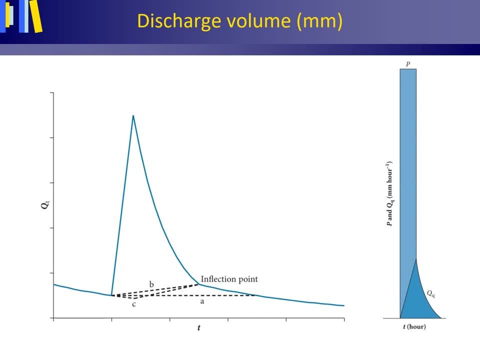 Multiplying this result by thousand millimeter per meter of course delivers an answer in millimeter. One should divide by the total drainage area, irrespective of the fact whether all or only part of the drainage basin actually contributes to the discharge. This is because the same total drainage 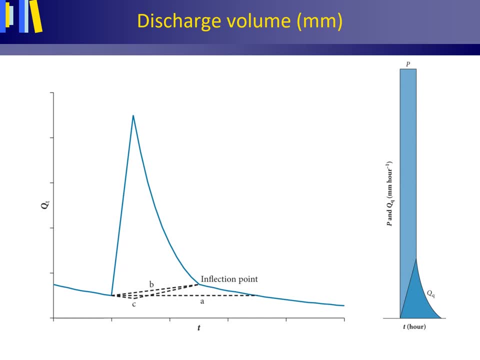 basin area is involved when translating precipitation or evaporation from volume units to length units or vice versa. Importantly, thus, a discharge presented, for instance, in millimeter per hour is not a velocity, what it may seem at the first glance, but a discharge in cubic. 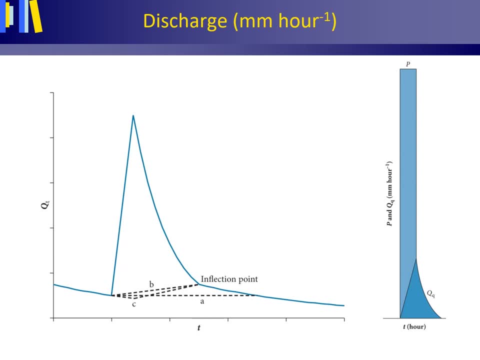 meter per hour, adjusted for the drainage basin area, by dividing by the total drainage basin area in square meter and multiplying by thousand millimeter per hour. The runoff coefficient of a stream can simply be determined by dividing the discharge volume in millimeter by the received precipitation volume, or. 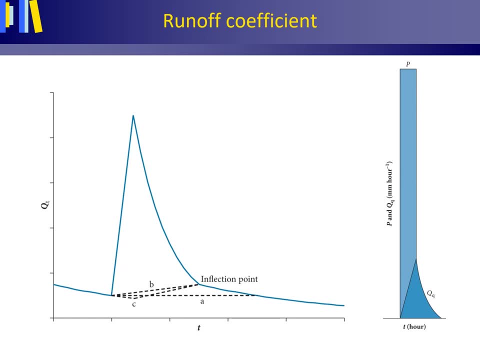 precipitation depth in millimeter and then multiplying by 100 to convert from fraction to percentage. The term runoff and runoff coefficient should be taken as the discharge of a stream. Another use of the term runoff is as a synonym for overland flow. Please note: the runoff coefficient on an annual basis is defined as the total. 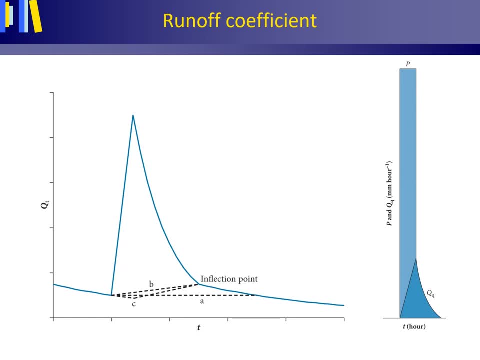 discharge volume in millimeter or cubic meter as a percentage of the precipitation volume in millimeter or cubic meter on an annual basis, whereas the runoff coefficient on a storm basis is defined as only the quick flow volume in millimeter or cubic meter as a percentage of the precipitation volume in millimeter or cubic meter on a storm basis. 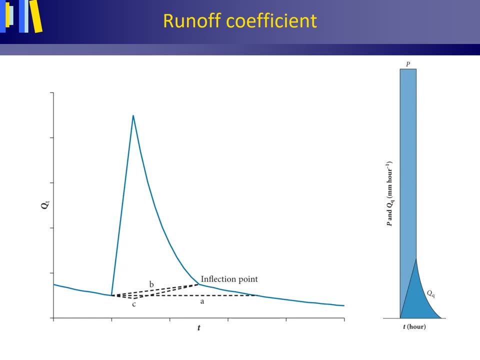 Usually in plots of storm hydrographs, discharge and precipitation are presented using different units, For instance cubic meter per second for discharge versus millimeter per hour for precipitation, And thus along differently scaled axes. The first impression of such figures may be that a large percentage of precipitation is discharged as quick flow during storms, which may be misleading. 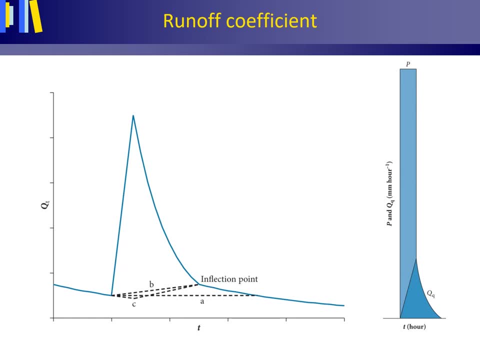 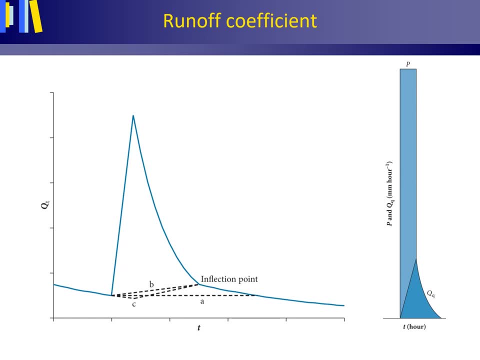 In situations when a small clay drainage basin is pre-wetted by earlier precipitation or when snow melts, storms with a high runoff coefficient may occur In a 파 Punchline. to get the perception right, the figure on the right shows a hydrograph of quickflow for a storm with the runoff coefficient of 30%, with, just for once, precipitation and quickflow presented in mm per hour, thus along equally scaled axis. 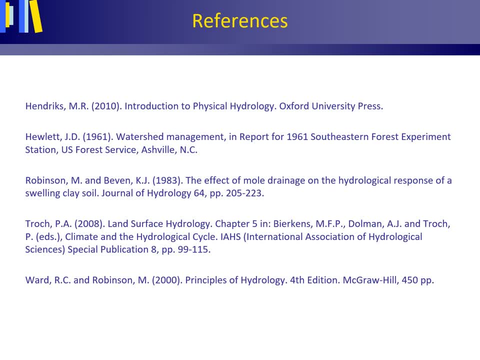 Part two of this lecture will be on hydrological simulation models. Thank you, 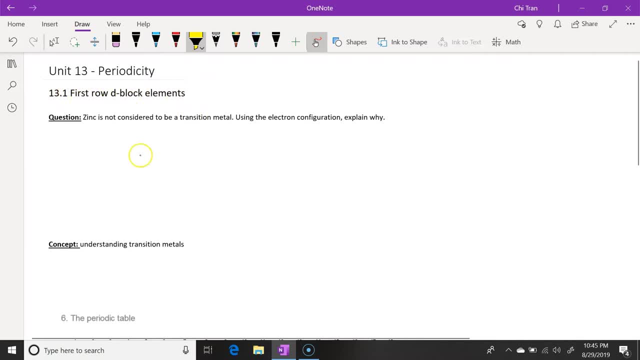 This video is about first row D, block elements. So the key word in the question is zinc is not a transition metal and we would need to use electron configuration in our answer And the concept of this question is understanding transition metals, So the definition of transition.